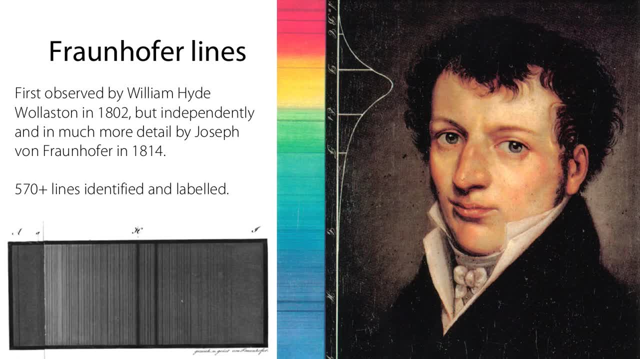 but Josef von Fraunhofer, working in Germany a few years later, did the first real scientific survey of these dark lines in the sun, these absorption lines as we now know they are. At the time they didn't know what they were and they were called in honor of him. he called them sun lines in German. 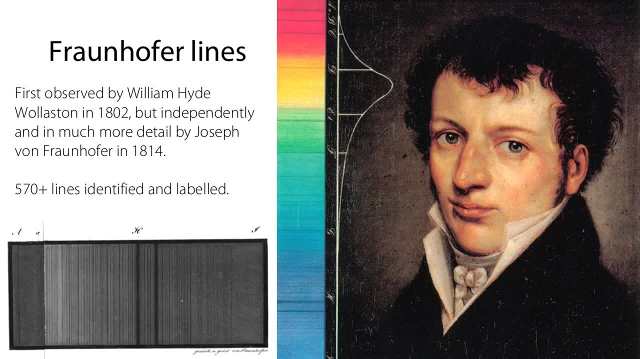 but we call them Fraunhofer lines in honor of the big guy himself. So here is a snapshot from his original report, His original plates, and you can see here this is part of the spectrum and this is grey- actually it would be yellow, I think, behind- and here are the prominent lines. 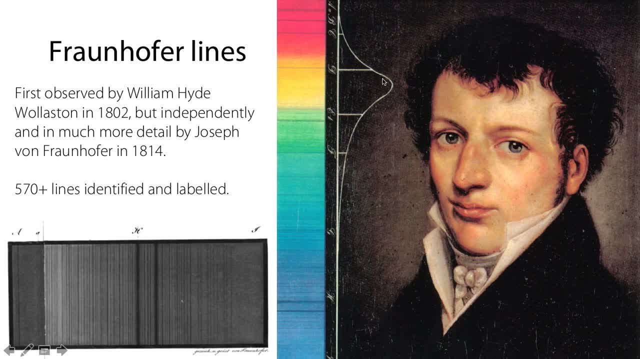 Here's a nice portrait of the man himself and you see the Planck curve here with certain lines marked, and here is a stellar spectrum with lines, although I have a suspicion it might be the wrong way around. I think red should have been down here, yellow here and blue up here. 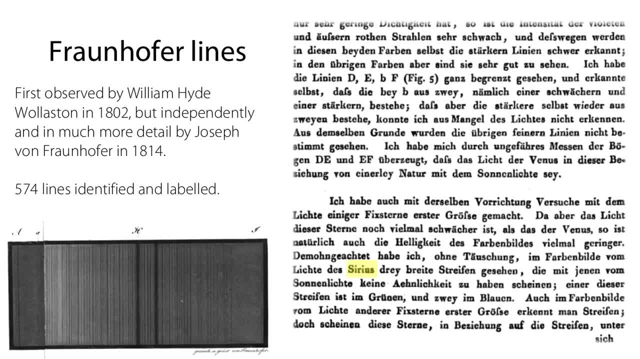 but it's just my sense. So yes, Fraunhofer observed the sun and he observed these sun lines, but he also- there you go, Sonnenlichter. he also did observe the stars. here he's made reference to lines of Sirius and he's also in this extract discussing Venus over here as well. 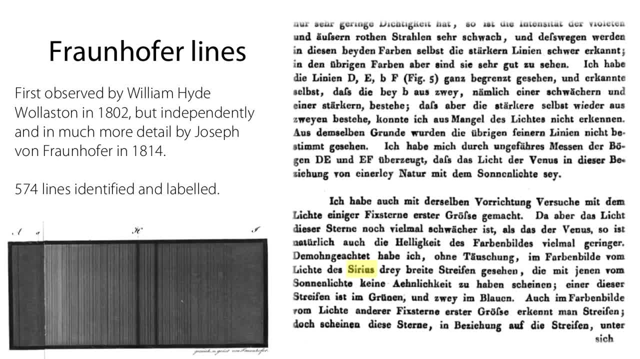 he's also discussing how the lines are different. So he was our first stellar spectrum, A stellar spectra getter, But he couldn't really, you know, he thought they were a curiosity and he was interested, but he didn't know what they were. he couldn't understand that. 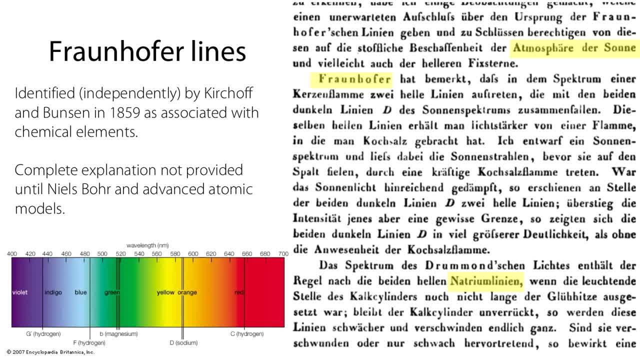 And that actually didn't happen for another 50 or 40 years or so. and Kirchhoff and Bunsen, also working in Germany in 1859, established by experiments that these were referred to as chemical elements. They did this in a laboratory, they knew about Fraunhofer lines and made the connection. 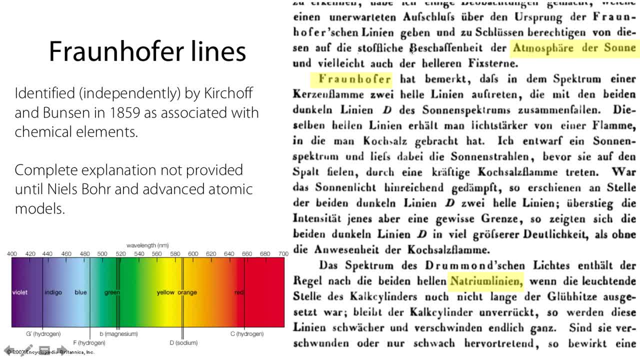 So here you see an extract from their report, a letter to the Berlin Physical Association. Fraunhofer and Atmosphäre der Sonne and Natrium Linien- Natrium you might not be familiar with in German, but you should be familiar with Na. 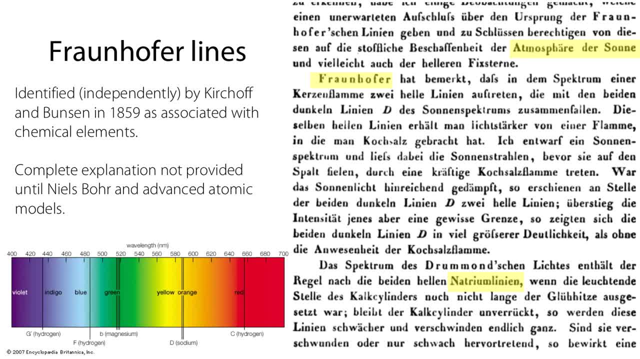 as an elemental syndrome. Natrium is Sodium, And so here again is a version of the spectrum and here are the elements, And Fraunhofer labelled the main lines by letters of the alphabet: G, F, little, b, big, D, C. 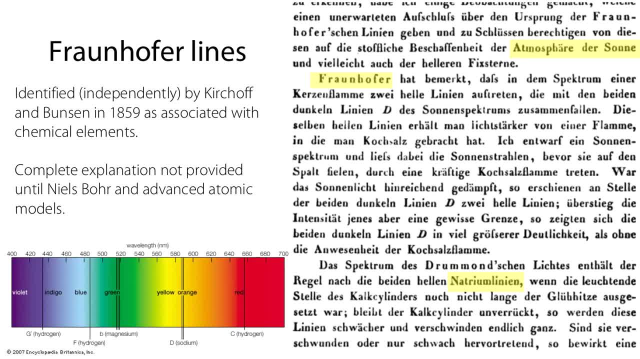 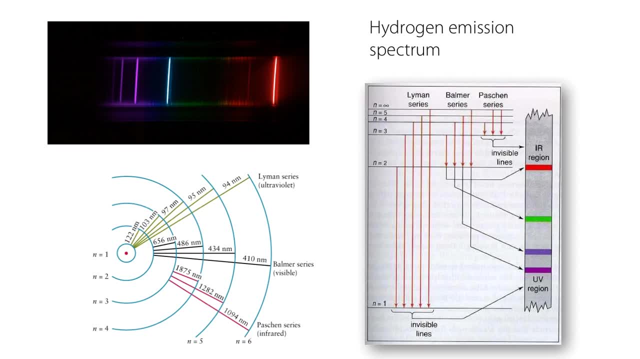 And although we now know much more what they are, this was Linien D der Sonnenspektrum. we now know that this is Sodium And we still call it the D line Bohr and later actually explained why these lines exist. 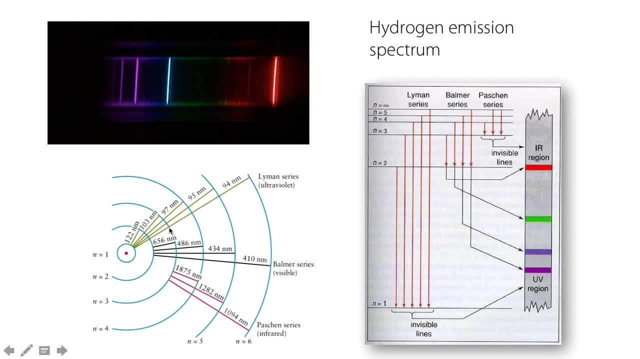 and they're all to do with electrons and electron transitions, But we don't actually, in this topic, really really need to know about that. What we just need to know is that these lines record the spectrum of a star. This is the visual of the spectrum from our own Sun. 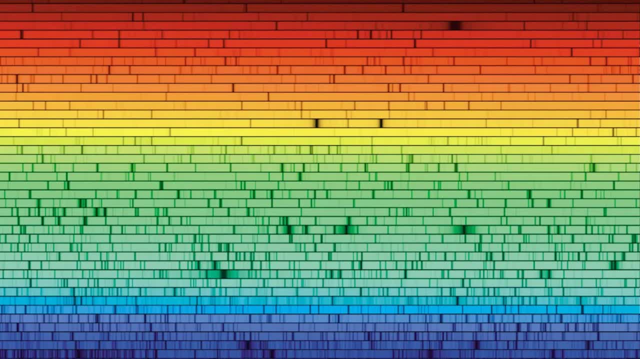 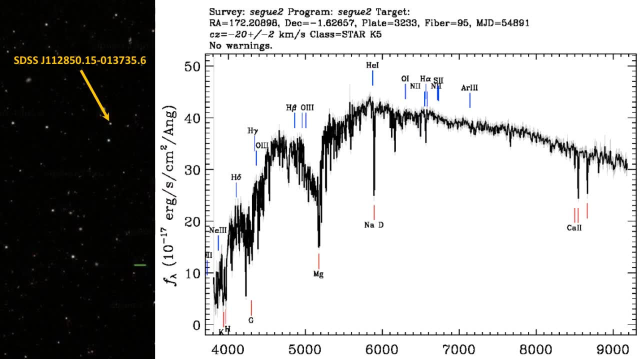 Imagine each of these rows taken out and then put in a big line and you'd see a very expanded version of our Sun's spectrum, which makes the lines much more obvious. We look at the stellar spectrum and you should recognise this slide from the previous lab. 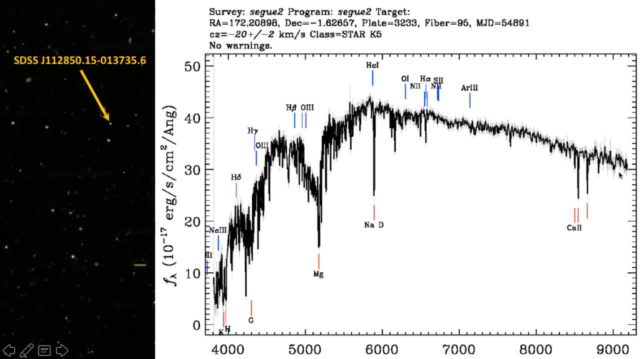 Again, here is the Planck curve, but superimposed on that is well, there's a lot of noise as well. this is a real-world experiment, but there are also deep gaps, corresponding to hydrogen, corresponding to magnesium, compared to sodium. 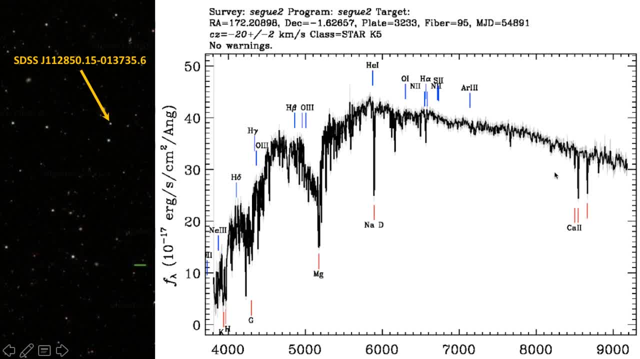 Remember, see that D Sodium, D line Compared to calcium, etc. etc. So that's what it looks like in a real star spectrum. So what we can tell from this is what the composition of that star is Technically. what we're looking at here is the star's atmosphere. 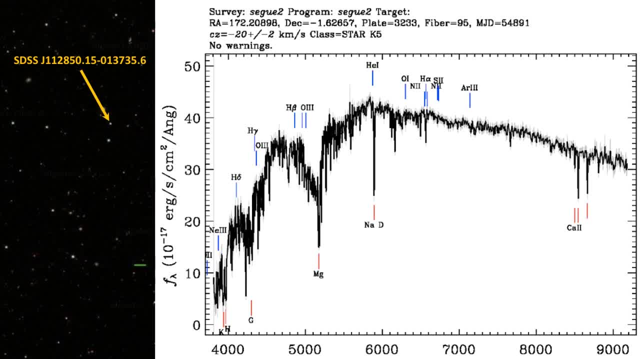 The photosphere of a star is the boundary of a star technically, where it becomes transparent or opaque and it gives off light at the boundary and that's the cause of our continuous spectrum And then shining through the stellar atmosphere is the. 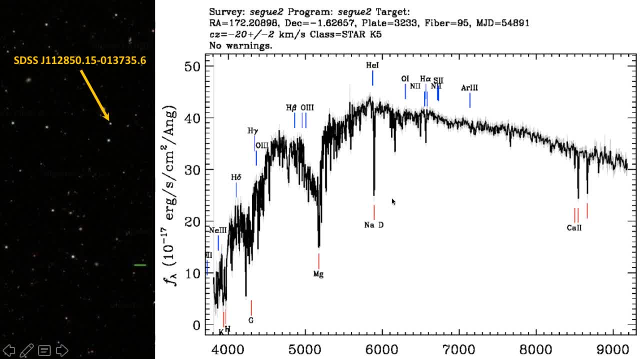 superimposed on it the lines from the elements present in the stellar atmosphere, In something as hot as our Sun or hotter. it is going to be just elements For fainter stars it could be, and often there's molecules. 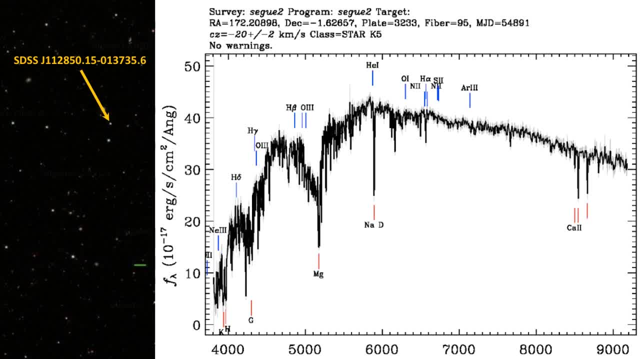 titanium oxide becomes very important as you get a lot colder. One other thing we do have to be a little bit aware of in real-world observations is that the interstellar medium, the space between stars, is not completely empty, And sometimes we have to be careful about. 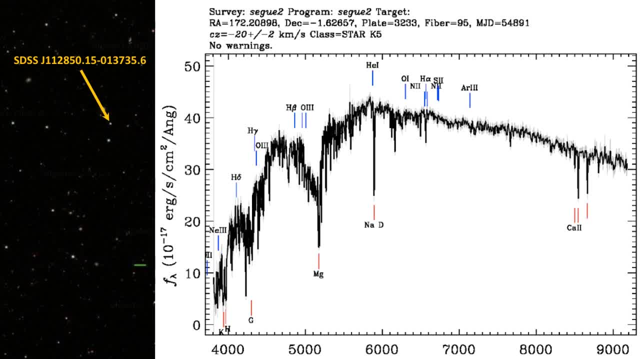 superimposed elements from that interstellar medium. Okay, Thank you very much. 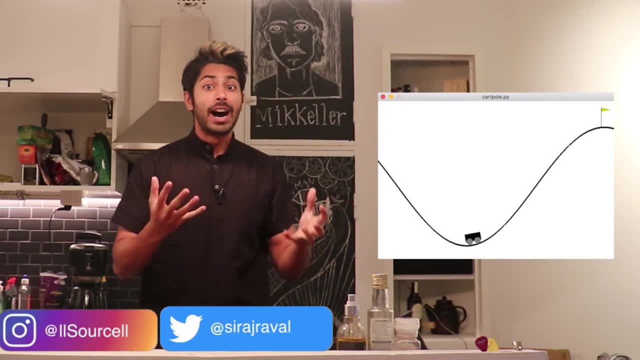 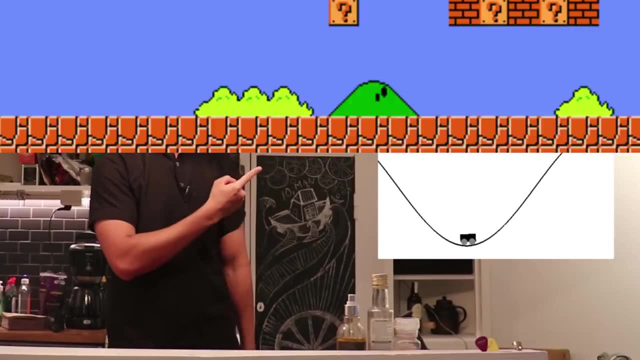 Hello world, it's Siraj, and let's see if we can teach an AI car how to drive to the top of a mountain using a super popular strategy called Q-learning. Since video games are considered virtual worlds, we'll want to use reinforcement learning. 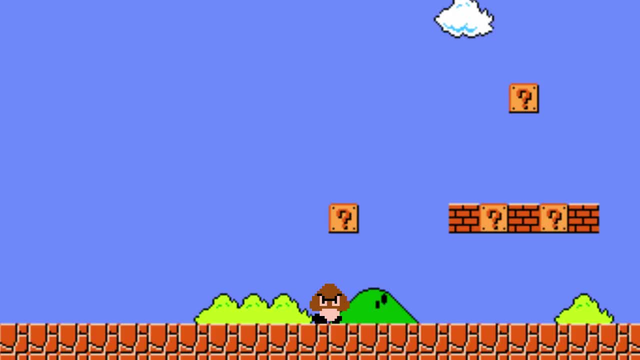 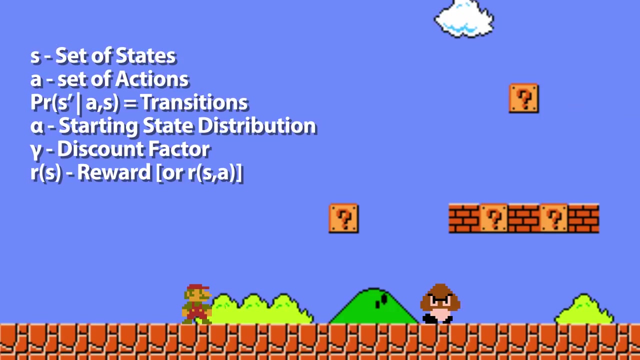 to help our AI learn how to best interact with its environment. That means using time-delayed labels, aka rewards, to help it learn how best to act in the environment through trial and error, to complete its objective. If an AI has a model of all the necessary elements of its environment, meaning the states. 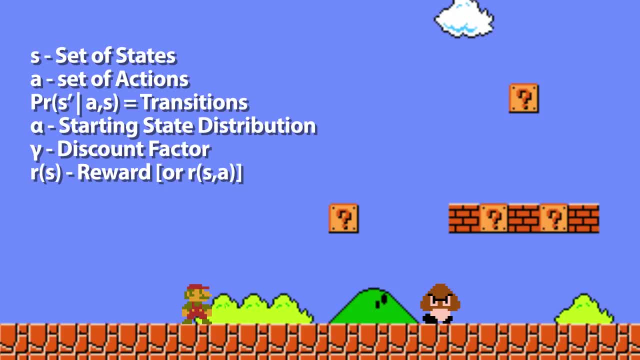 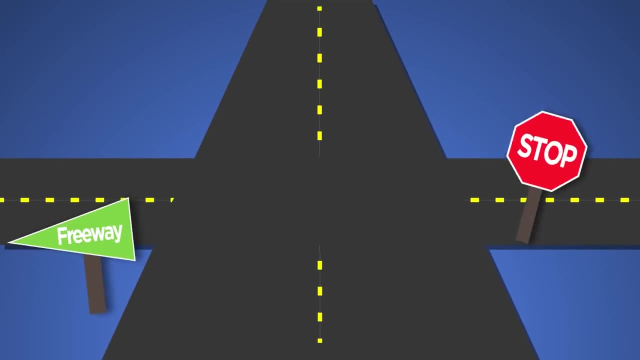 rewards, transition model, etc. basically everything that makes up a Markov decision process. it can easily then use a planning algorithm to compute a solution to whatever its objective is So easy a liberal arts major could do it. This is considered model-based learning.